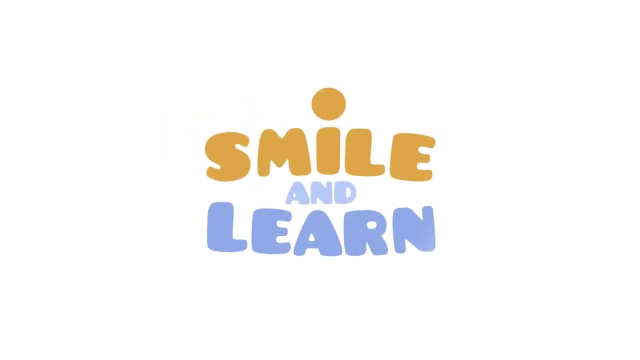 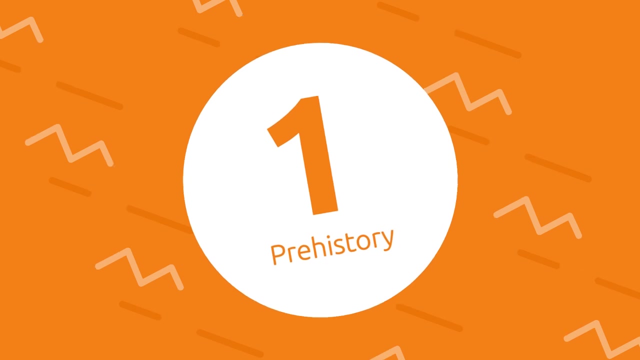 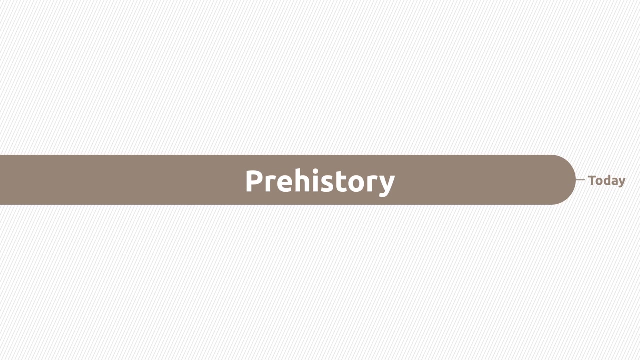 Five things you should know about prehistory. Prehistory marks the oldest period in the history of humanity. It begins with the appearance of human beings and ends with the invention of writing. This period started five million years ago. Yes, you heard right, It was ages ago. It's called prehistory because it refers 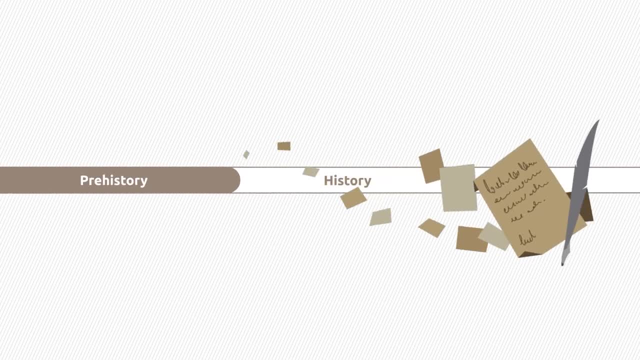 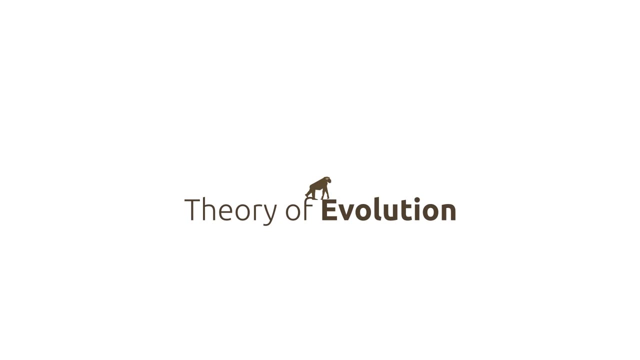 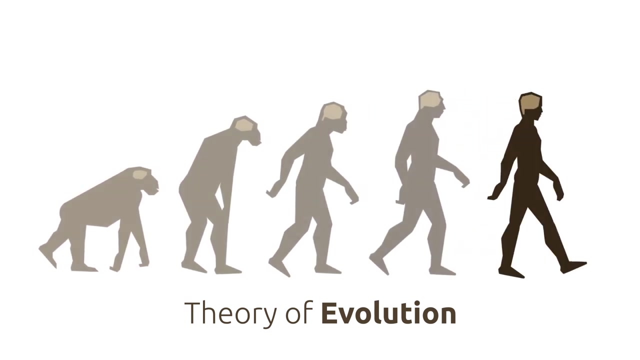 to the time before history, meaning before the invention of writing. According to the theory of evolution, modern humans- meaning us- evolved from a certain group of primates who were able to stand upright on their legs. Their brain grew in size and this allowed them to be able to think. 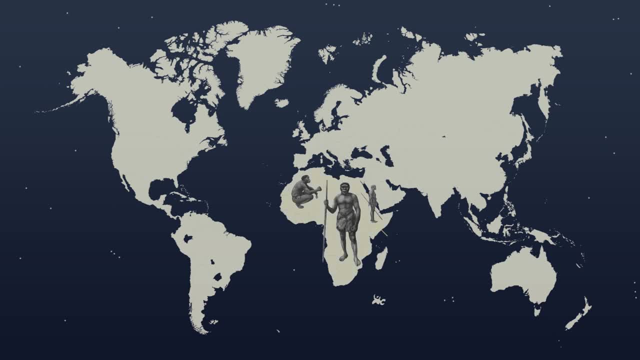 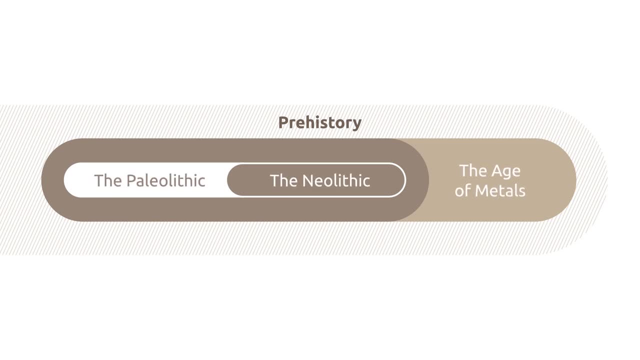 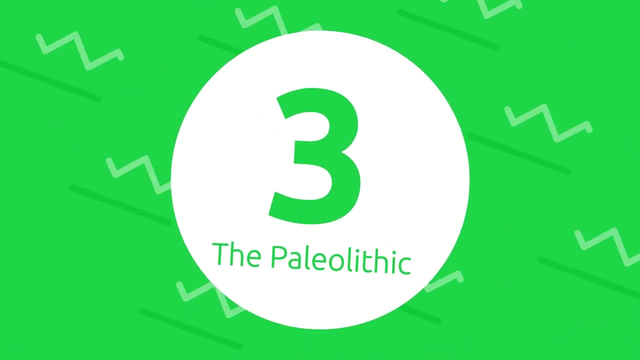 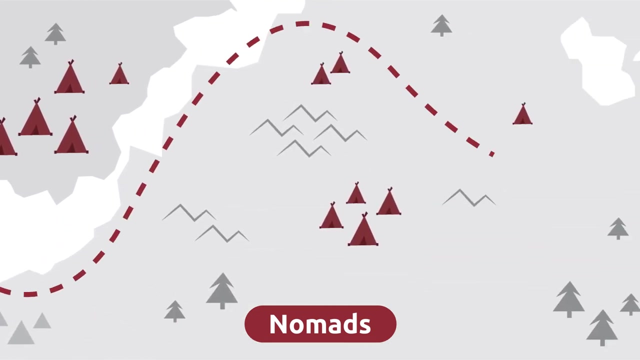 Did you know that the first humans lived in Africa? We divide prehistory in three periods: the Paleolithic, the Neolithic and the Age of Medals. During the Paleolithic period, humans were nomads, meaning they didn't settle in the 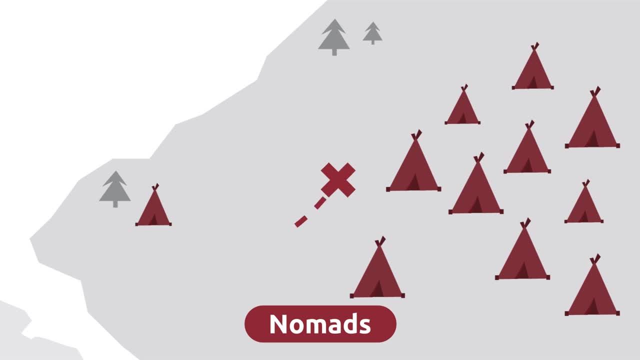 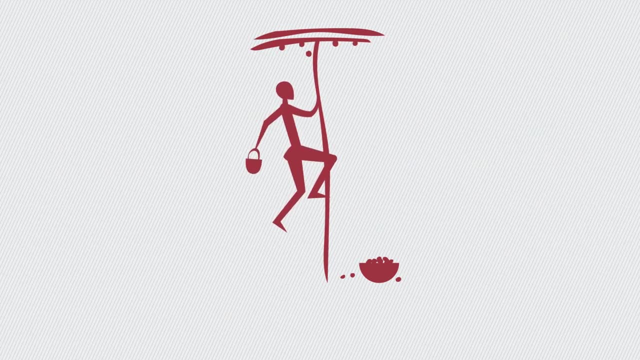 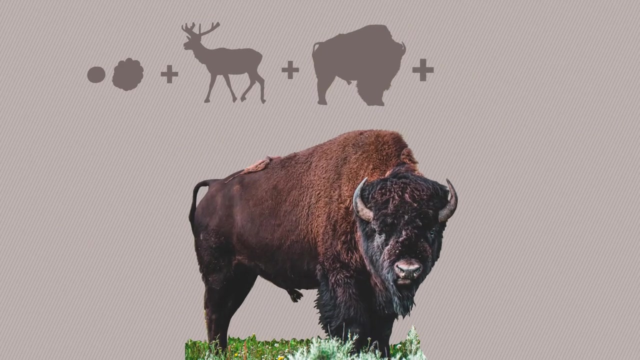 same place. They traveled from one area to another looking for a location to fish, to hunt or collect food. Yes, you heard right: They were hunters and collectors. Among their favorite foods were wild berries, deer, bison or even mammoths. 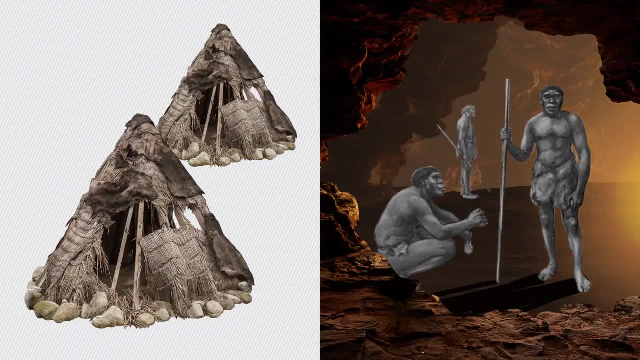 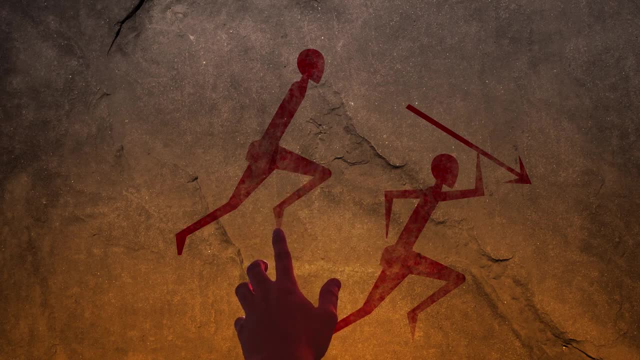 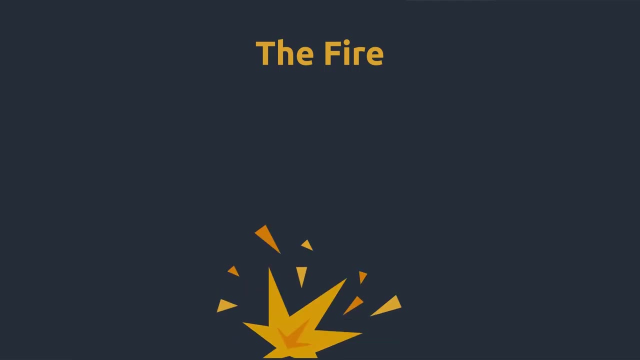 They lived in tribes, dwelling huts or natural caves that they decorated with their well-known cave painting. They represented hunting scenes like the one you can see in this picture. Isn't it incredible that their art still remains to this day? Fire was discovered in Paleolithic times and humans made their first stone tools. 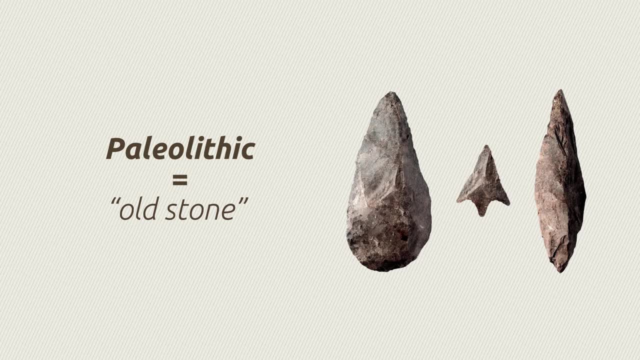 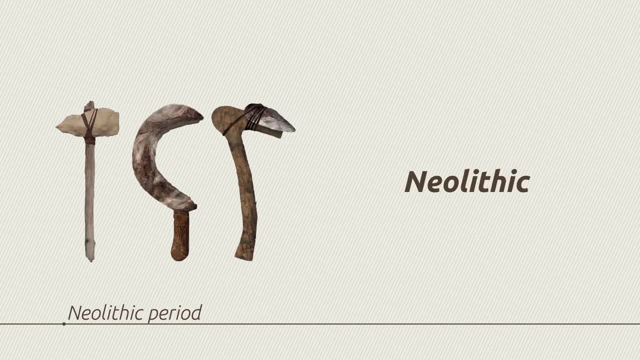 This is where the word comes from. Paleolithic means old stone. Those first men were progressing and perfecting their tools. This is how the Neolithic period was initiated. The word Neolithic means new stone. Neolithic times began ten thousand years ago. 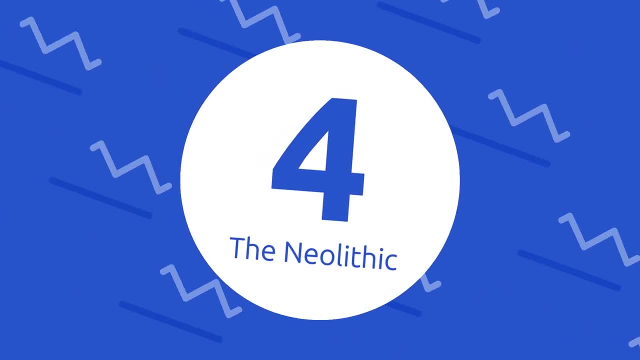 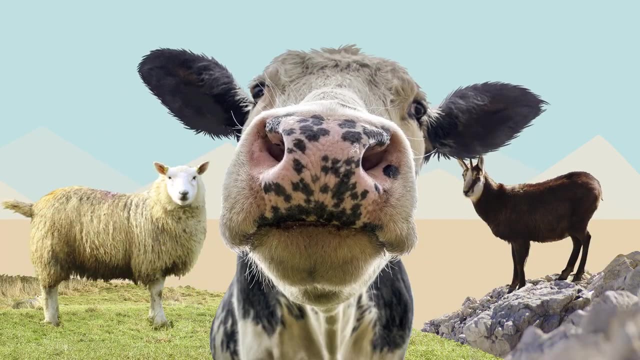 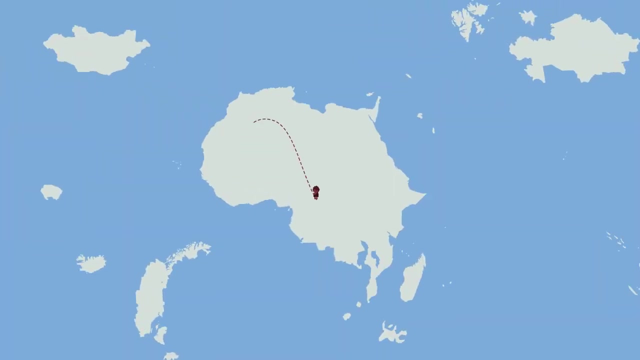 10. What was Neolithic? Let's take a look. How was it created? Neolithic times began with the practice of agriculture and cattle raising. During this time, human beings started domesticating animals and cultivating the land to grow food. For this reason, they stopped being nomads and their lifestyle became sedentary. 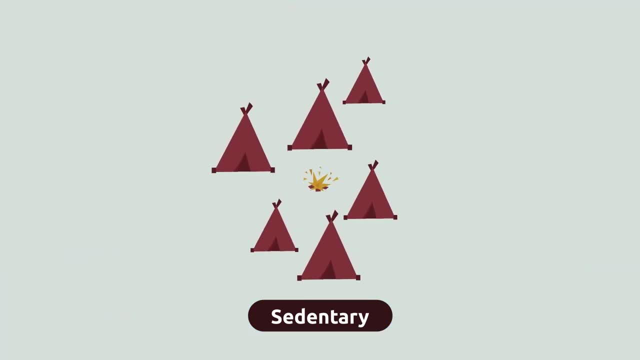 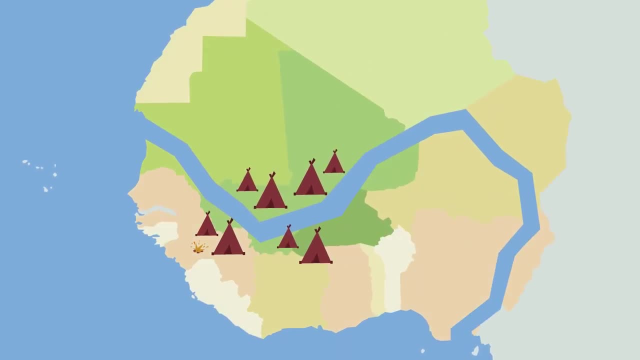 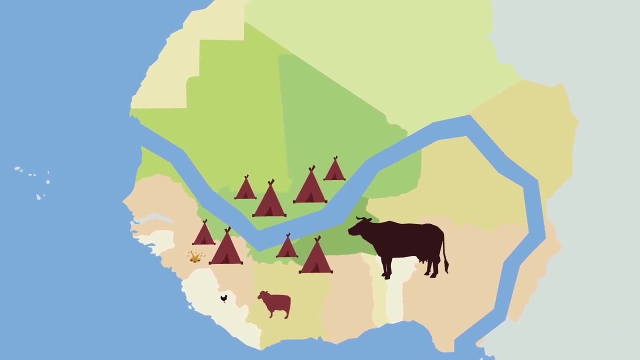 They didn't have to travel to look for food. They had everything they needed in their villages. Neolithic times are marked by the first settlements found near fertile land where there was plenty of water. They needed water for their animals and crops. Cattle raising and cultivating the land improved their diet. 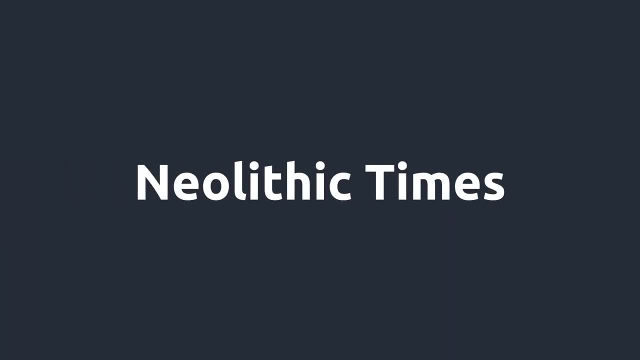 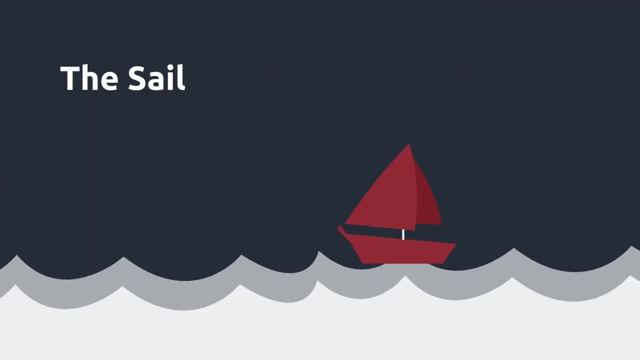 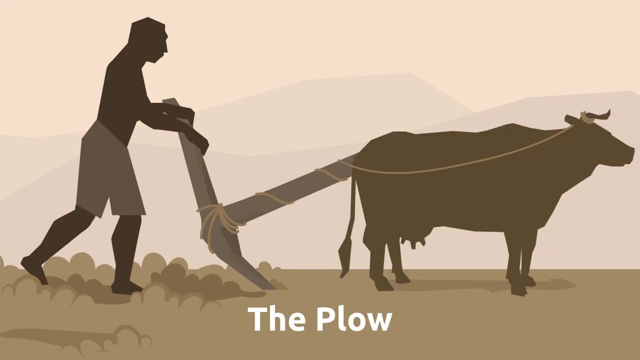 That's why populations started to grow. During this time, an important discovery came about – the wheel. It made things easier for agriculture. The invention of other extraordinary things like the sail, the loom, the plow or pottery also took place. 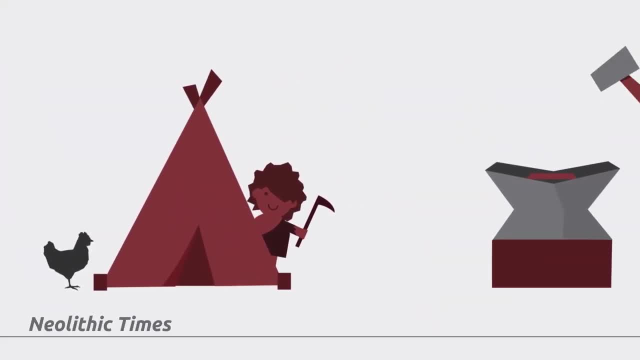 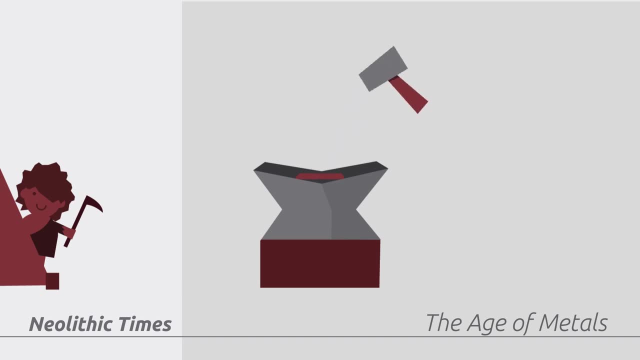 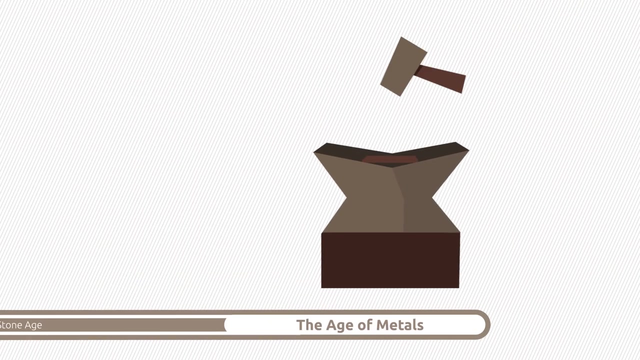 Human beings continued growing, They started progressing and they started using weapons and metal tools. This is the moment Neolithic times end and the Age of Metals begins. The Age of Metals was a revolutionary time because metal tools were more wear-resistant than stone tools. 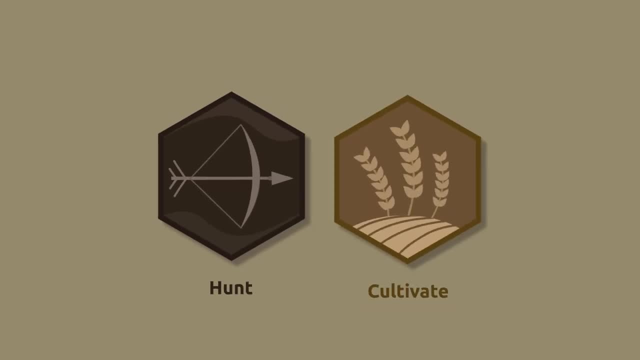 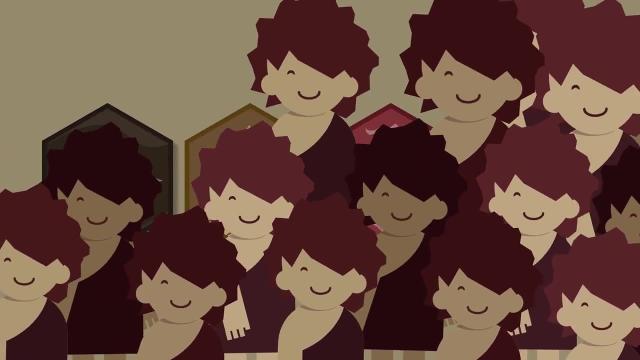 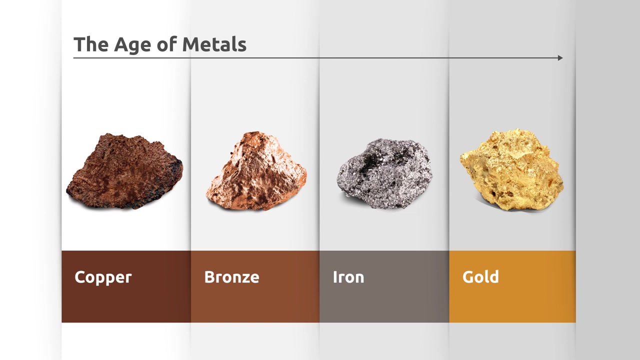 These new gadgets allowed men to hunt and cultivate the land more easily. This improvement in farming and agriculture- The decline in agriculture- resulted in having more food. That's why population increased. Metals like copper, bronze, iron or even gold were discovered during this time. 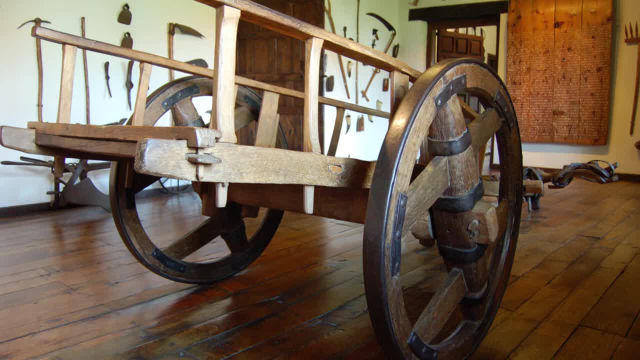 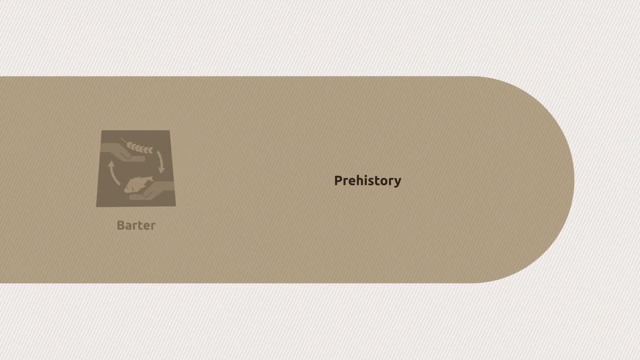 Craftsmanship and transportation improved a lot. This gave rise to commerce and the trading of products. This system is known as barter. Prehistory ended with the invention of writing. That is a fascinating period, Don't you think so? Thank you for watching. 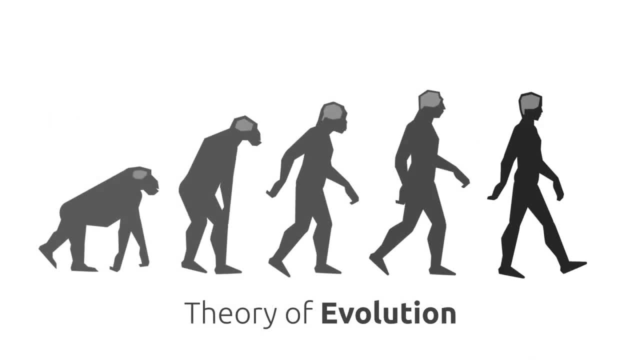 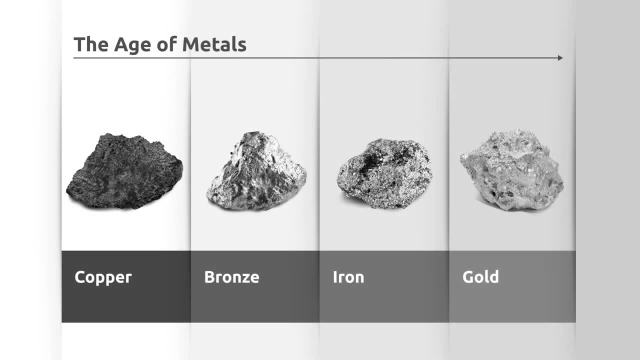 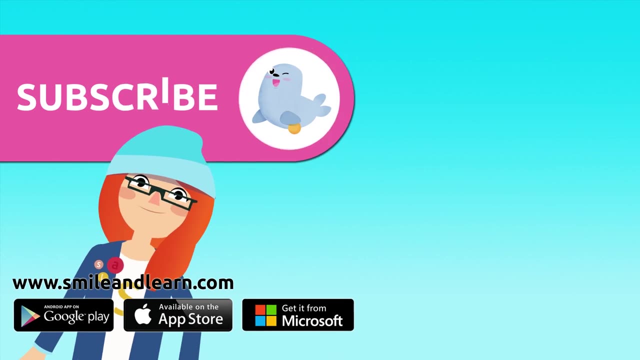 Please like and subscribe. These are the five things you should know about prehistory. Did you like learning about them? Thanks for watching.